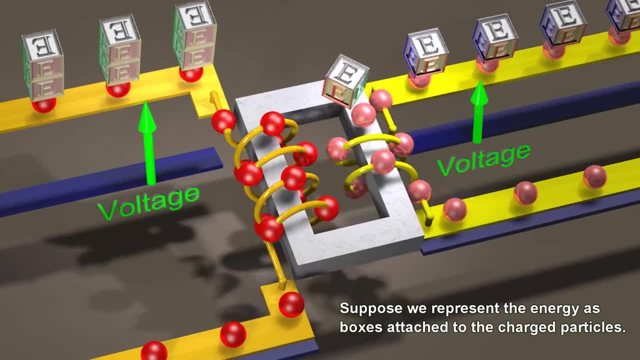 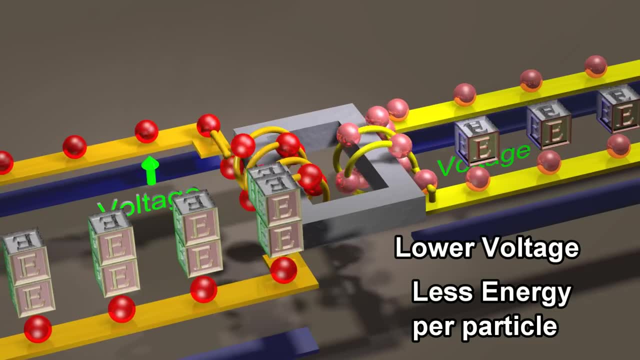 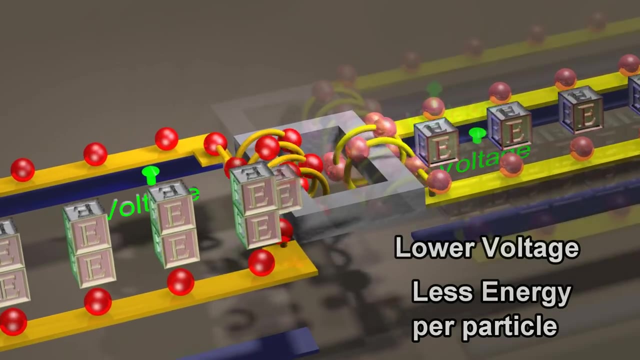 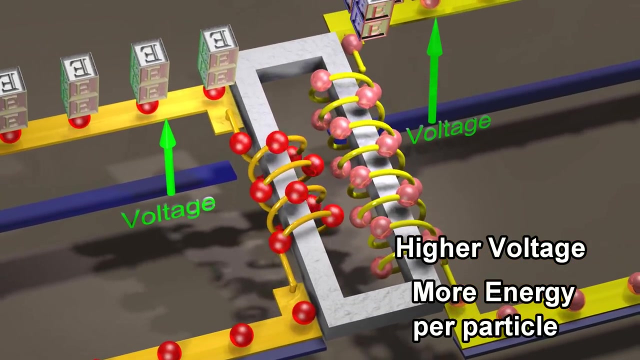 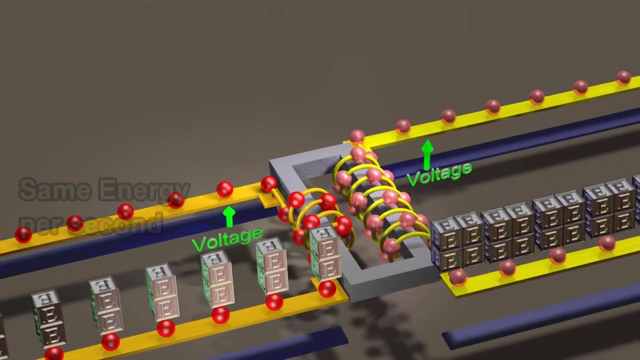 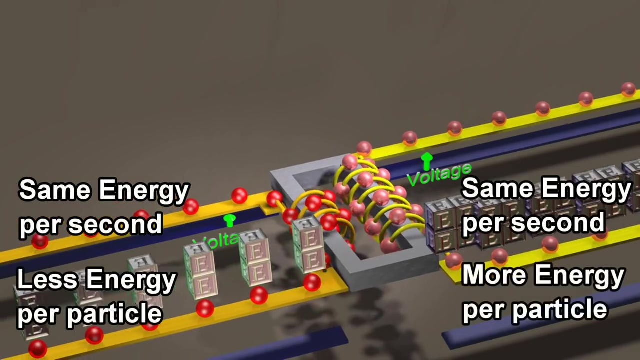 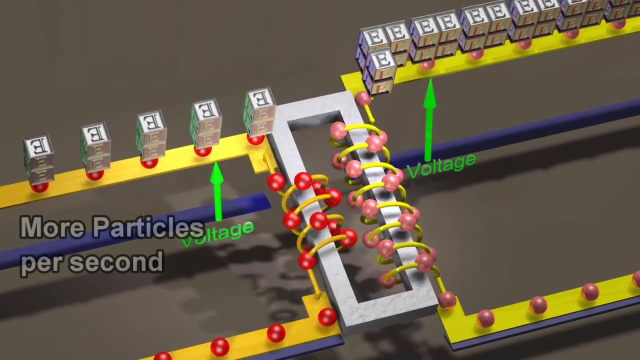 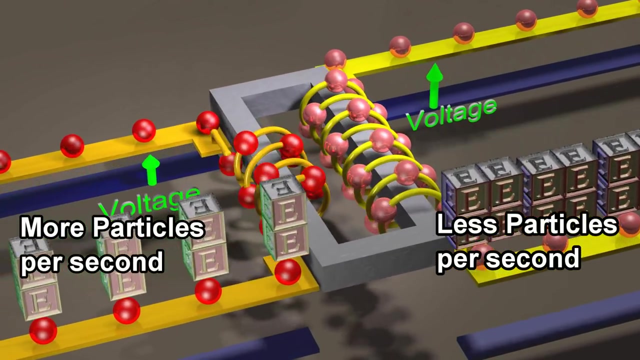 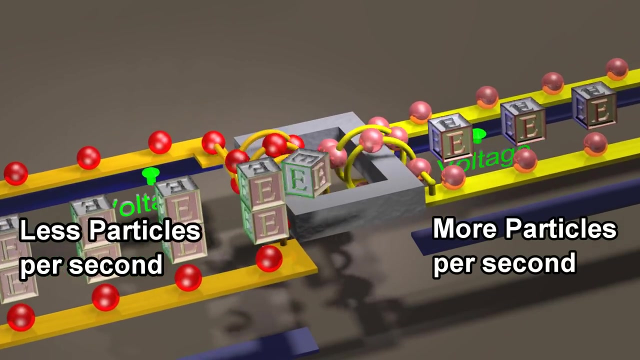 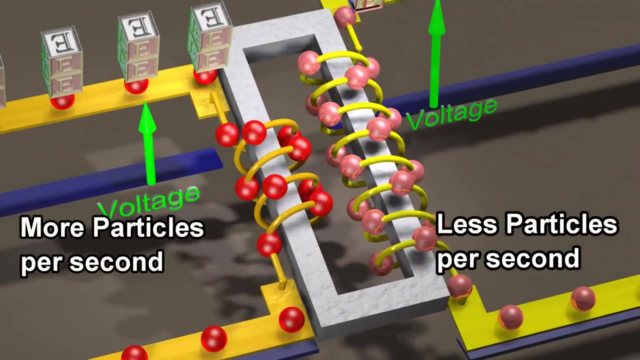 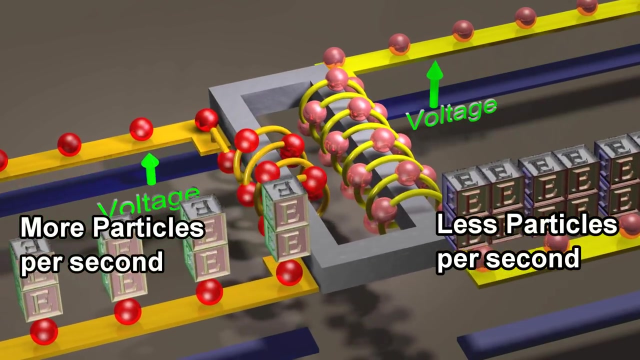 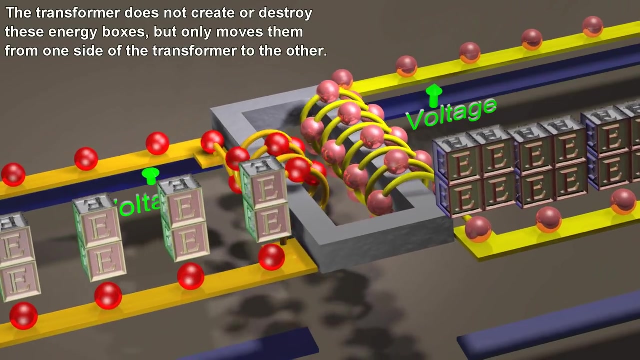 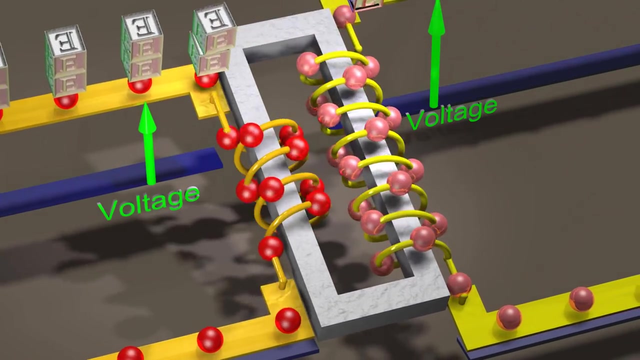 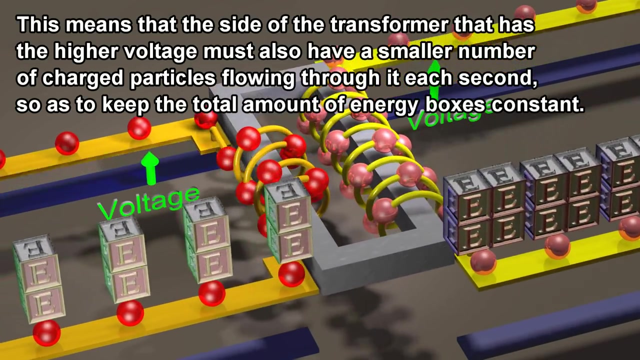 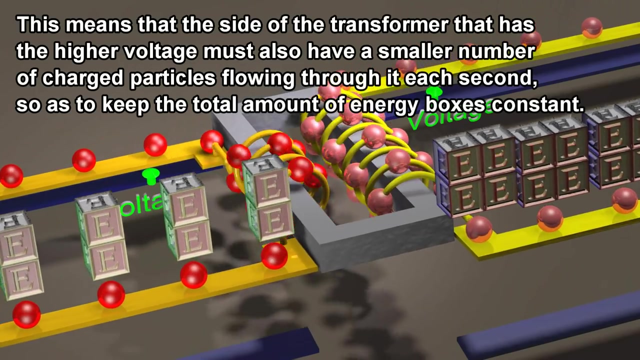 Suppose we represent the energy as boxes attached to the charged particles. Thank you for watching. Thank you for watching. A transformer that has the higher voltage must also have a smaller number of charged particles flowing through it each second, so as to keep the total amount of energy boxes constant. 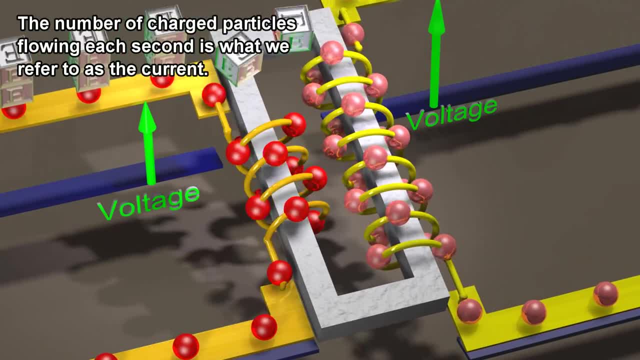 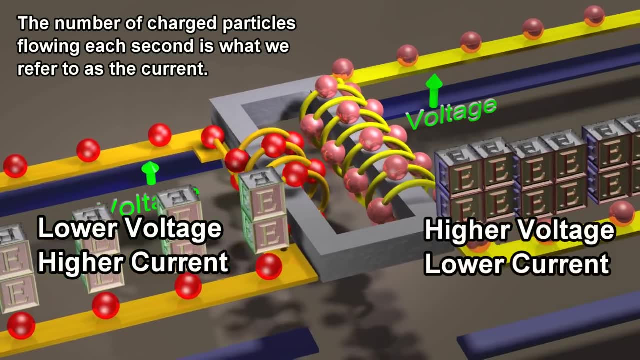 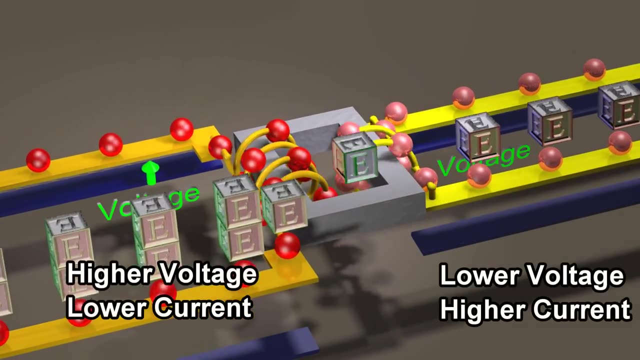 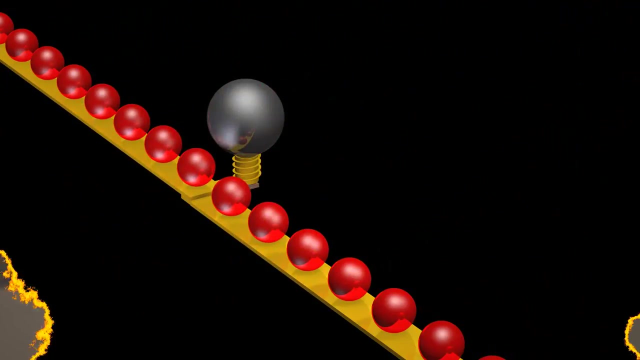 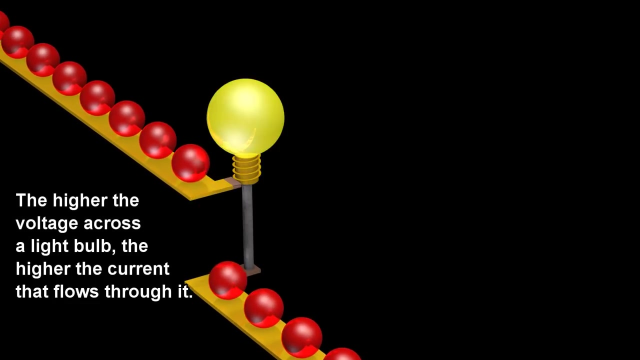 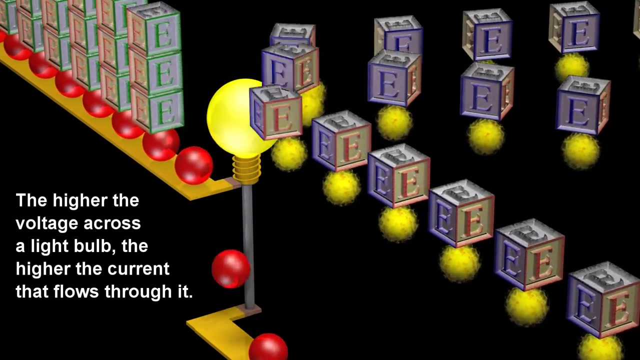 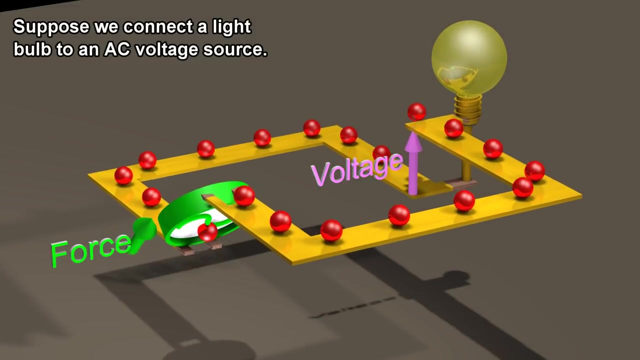 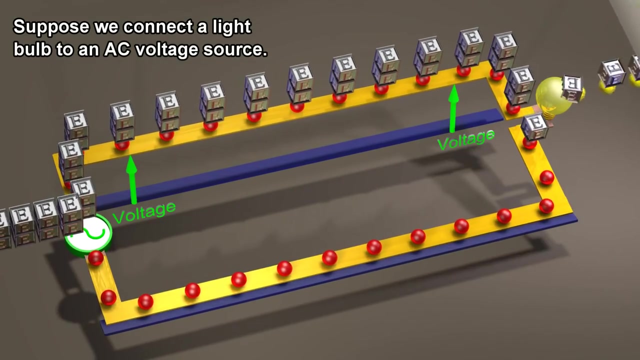 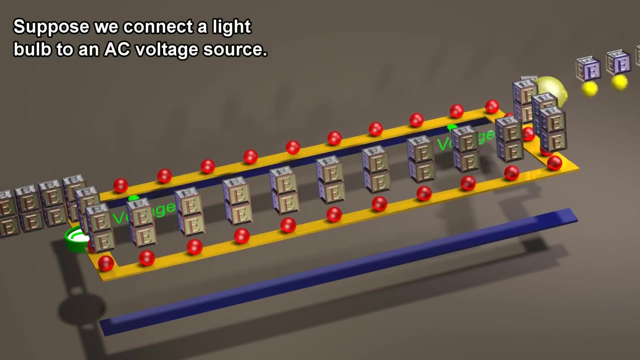 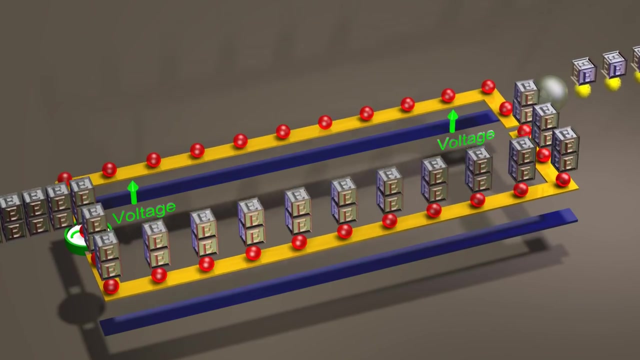 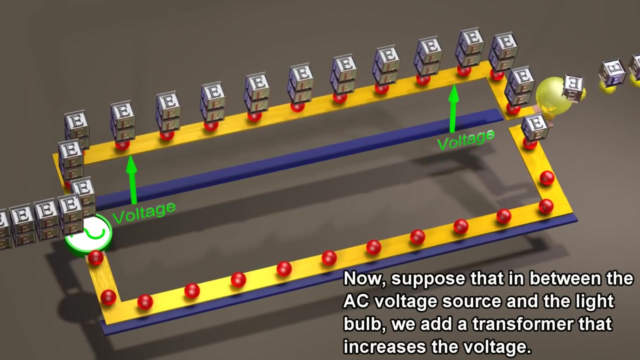 The number of charged particles flowing each second is what we refer to as the current. The higher the voltage across a light bulb, the higher the current that flows through it. Suppose we connect a light bulb to an AC voltage source. Now suppose that in between the AC voltage source and the light bulb we add a transformer that increases the voltage. 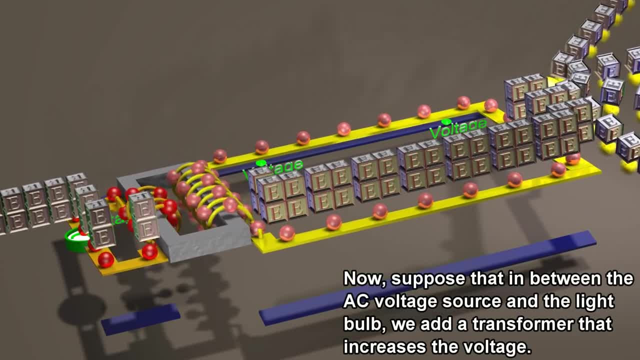 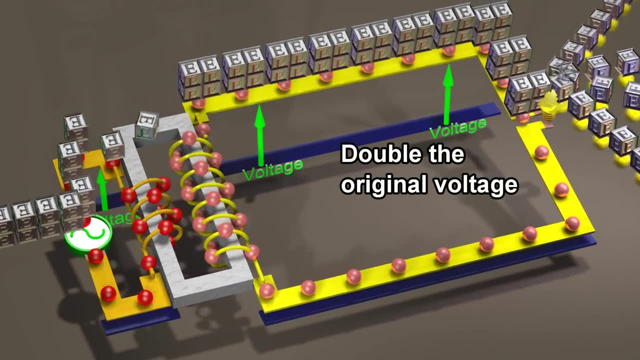 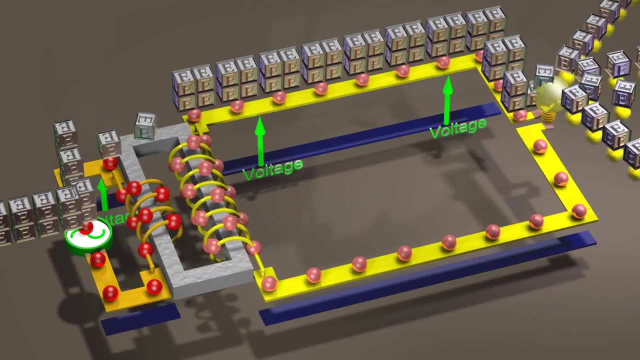 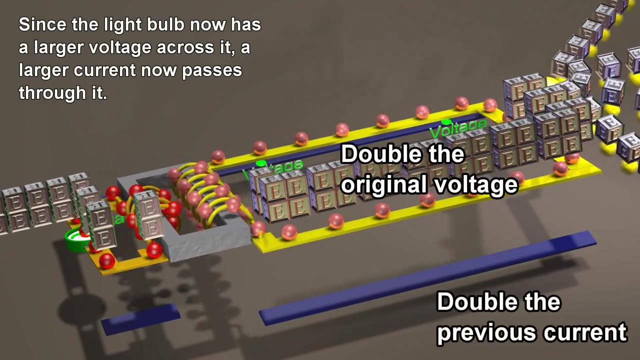 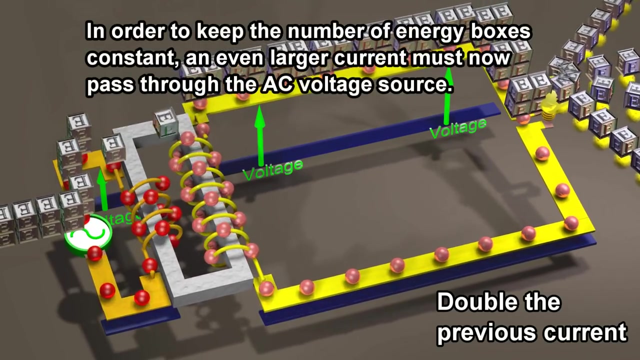 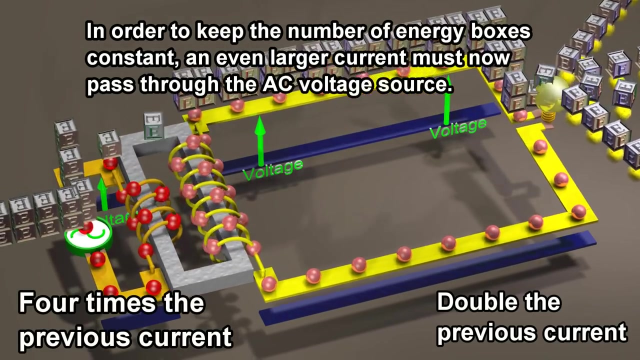 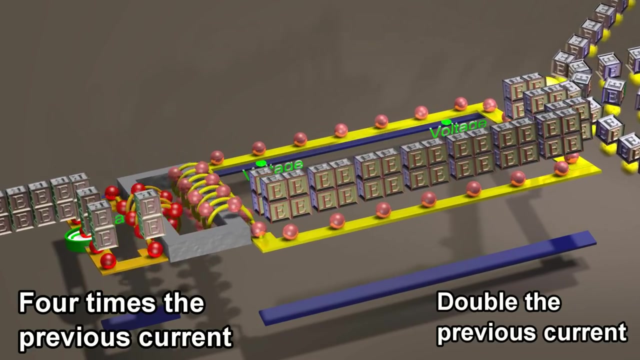 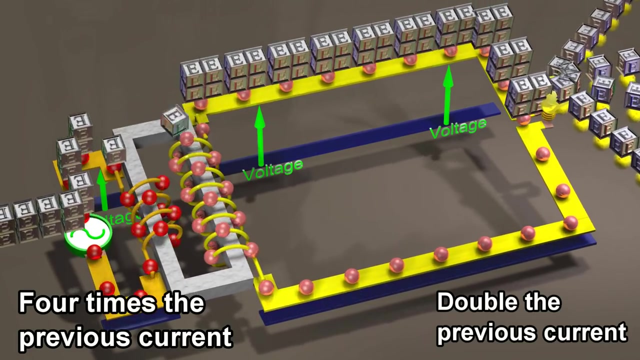 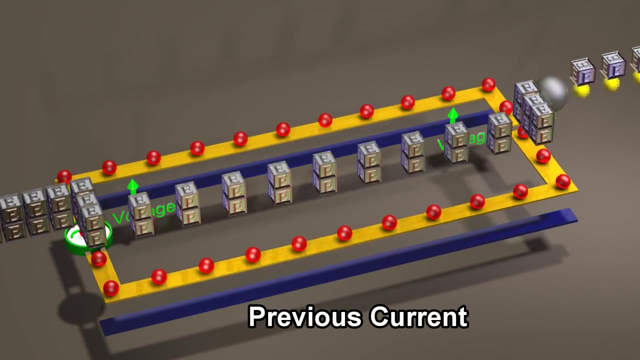 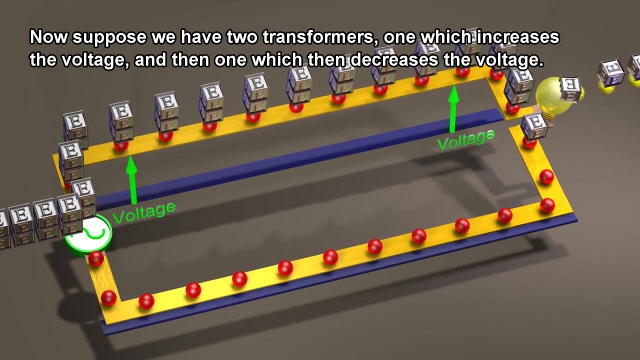 Since the light bulb now has a larger voltage across it, a larger current now passes through it. In order to keep the number of energy boxes constant, an even larger current must now pass through the AC voltage source. Now suppose we have two transformers, one which increases the voltage and then one which decreases the voltage. 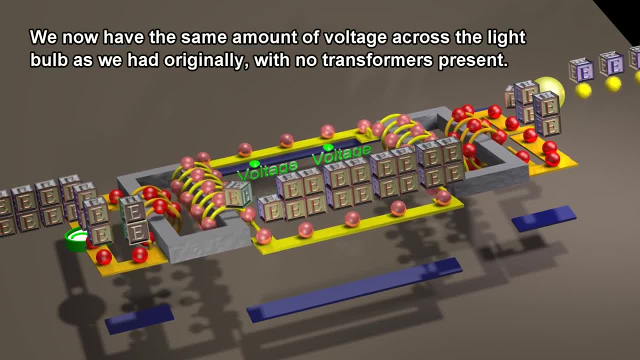 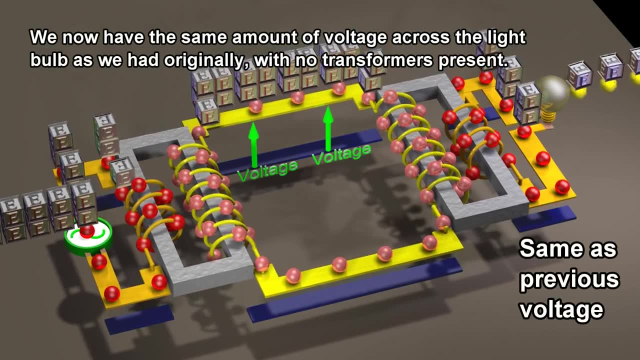 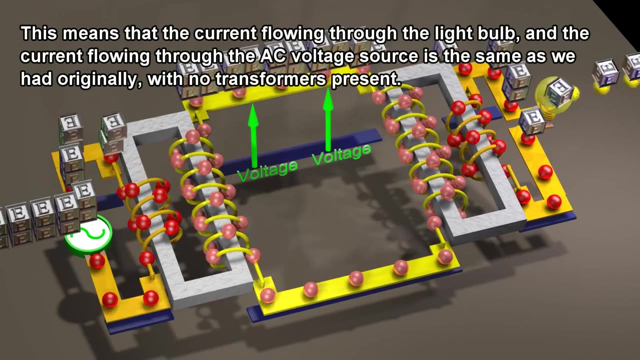 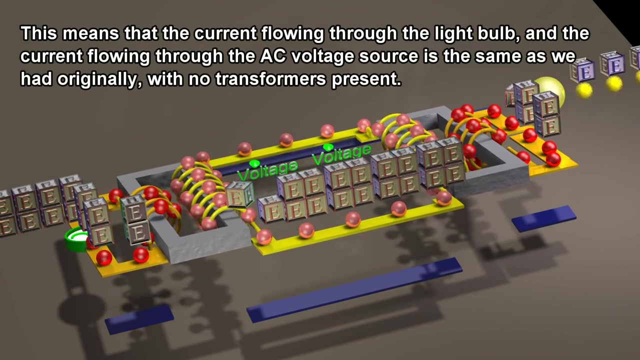 We now have the same amount of voltage across the light bulb as we had originally with no transformers present. This means that the current flowing through the light bulb and the current flowing through the AC voltage source is the same as we had originally with no transformers present. 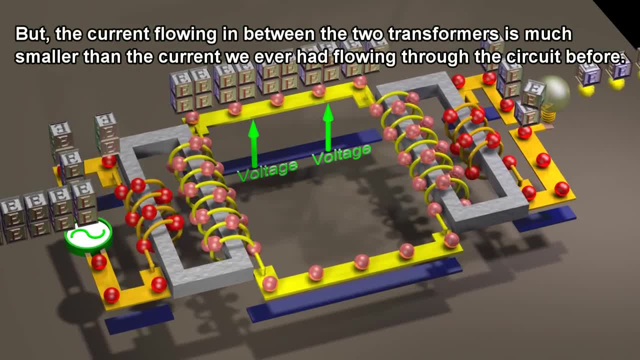 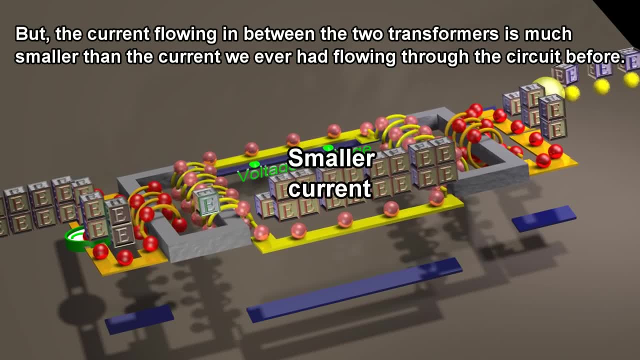 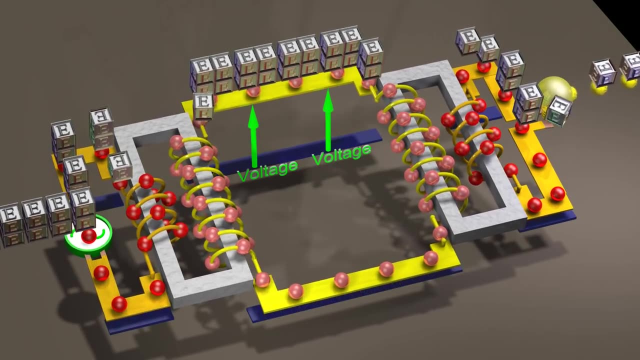 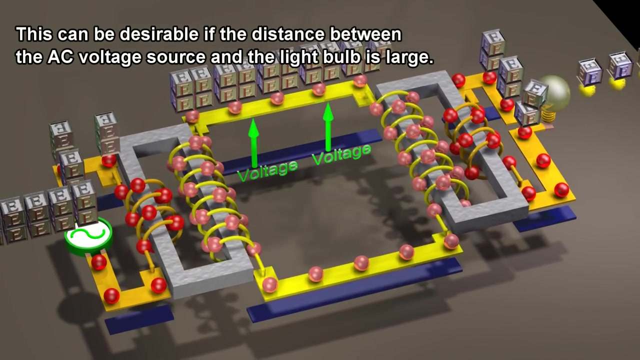 But the current flowing in between the two transformers is much smaller than the current we ever had before. But the current flowing in between the two transformers is much smaller than the current we ever had before flowing through the circuit before. This can be desirable if the distance between the AC voltage source and the lightbulb is large. 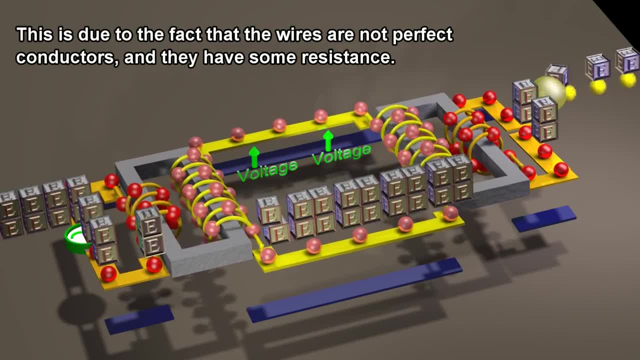 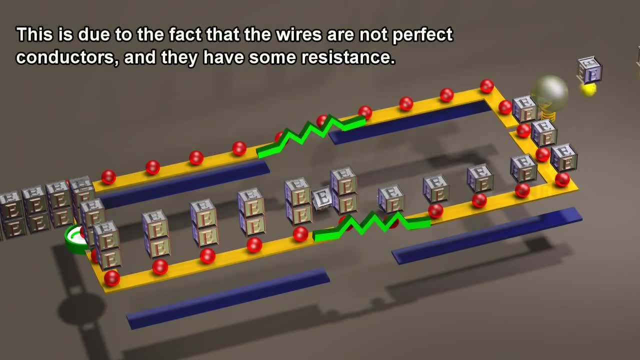 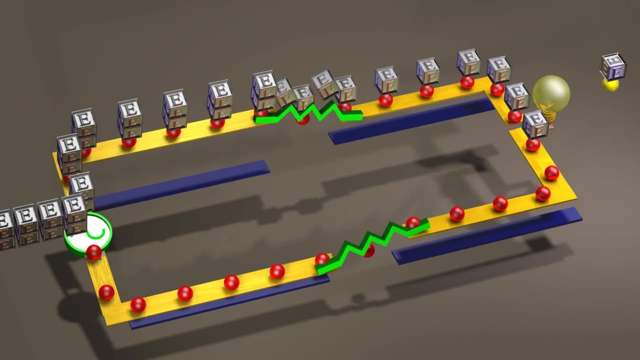 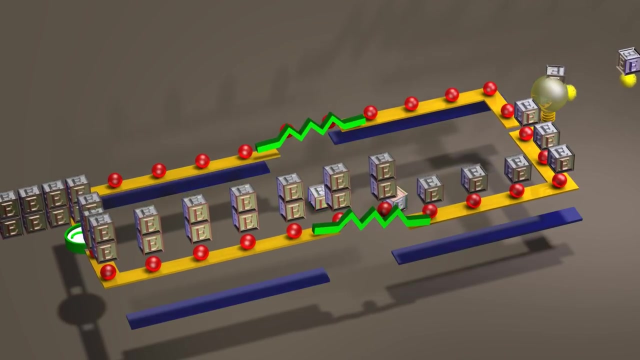 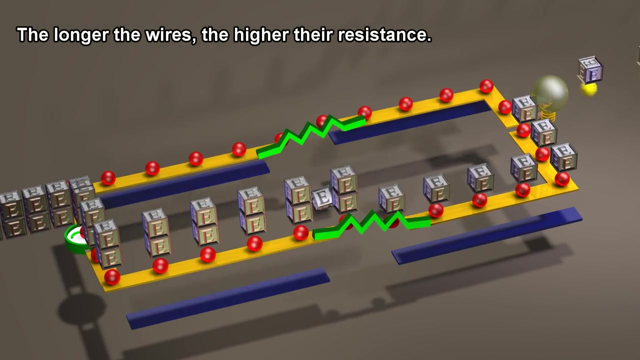 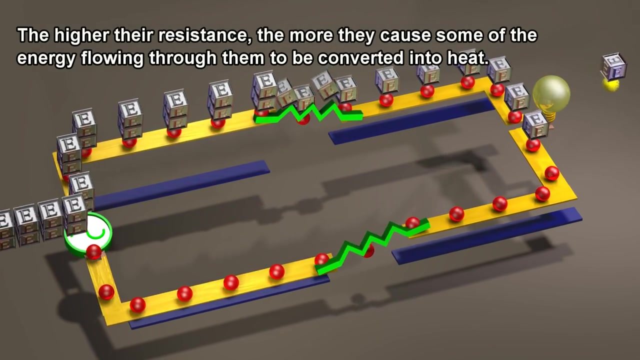 This is due to the fact that the wires are not perfect conductors and they have some resistance. The longer the wires, the higher their resistance. The higher their resistance, the more they cause some of the energy flowing through them to be converted into heat. 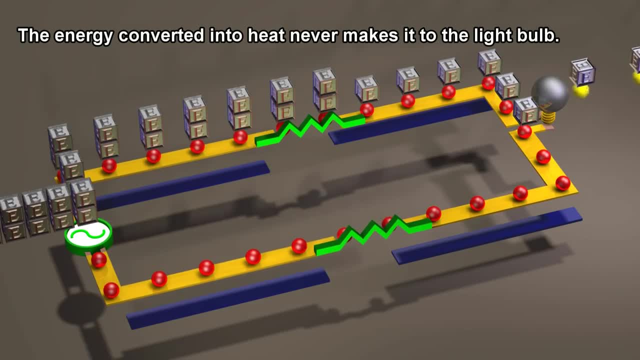 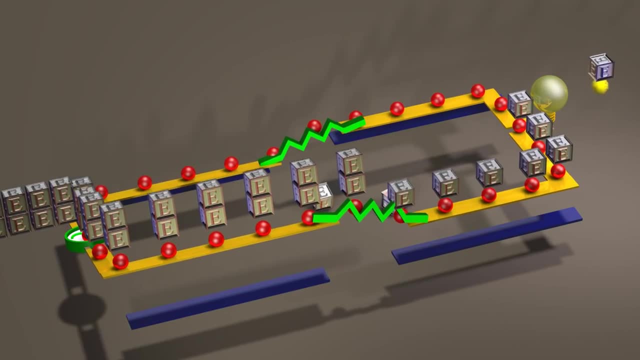 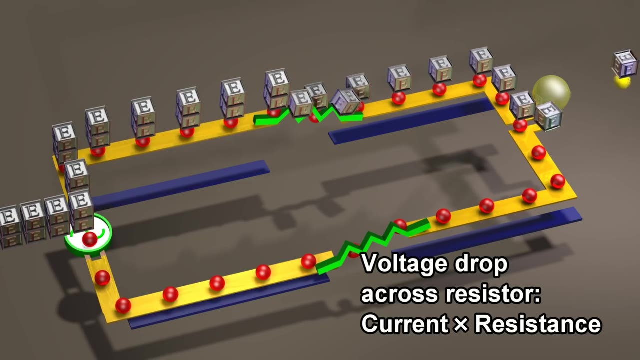 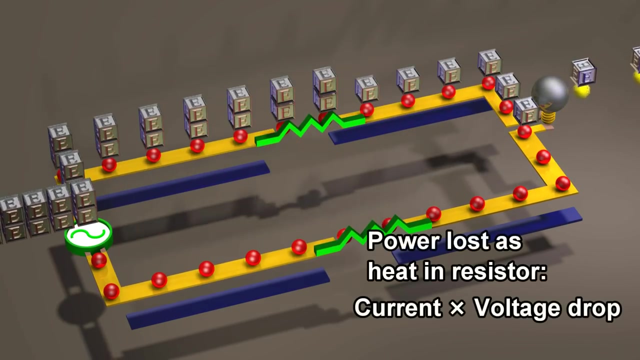 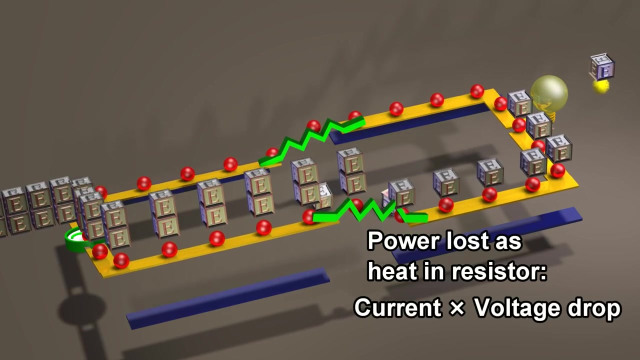 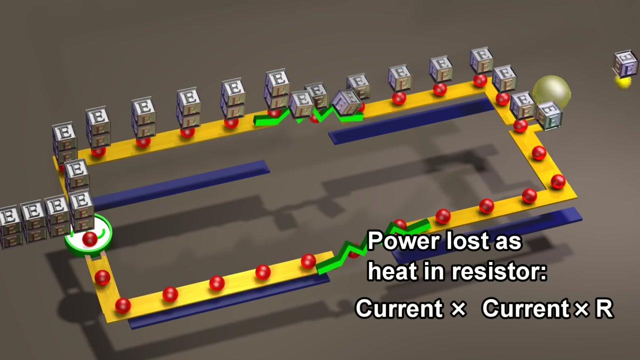 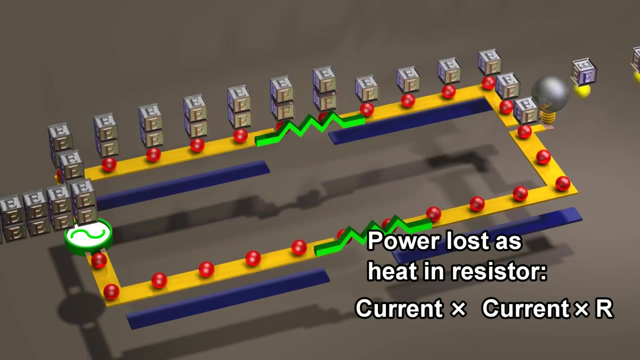 The energy converted into heat never makes it to the lightbulb. Listen and see to what extent the connection is working, The strength of the wires and the power of theüm meter. Guest said him that radio didn't work because the idea is no force to let go. 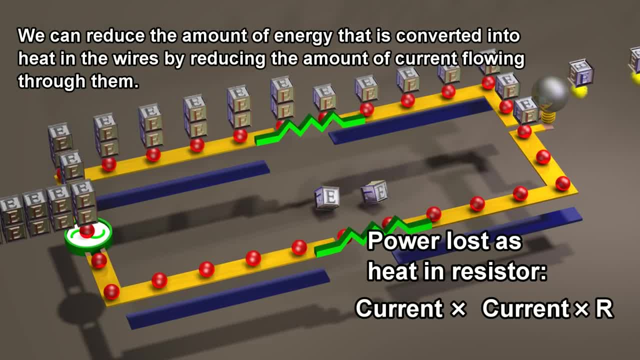 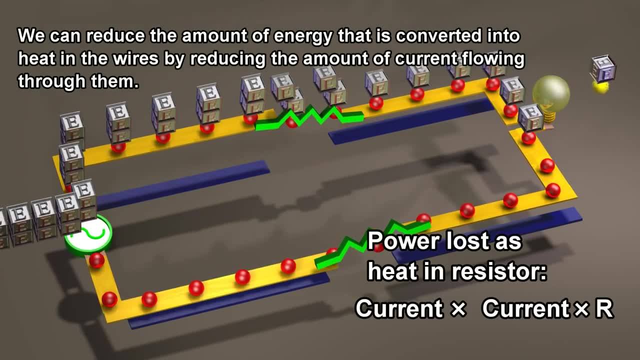 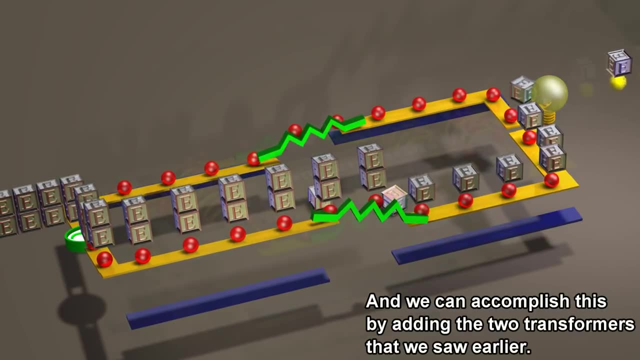 He said, radio wasn't allowed to play songs on a 핏h İon precedent to convert it into heat in the wires by reducing the amount of current flowing through them, And we can accomplish this by adding the two transformers that we saw earlier. 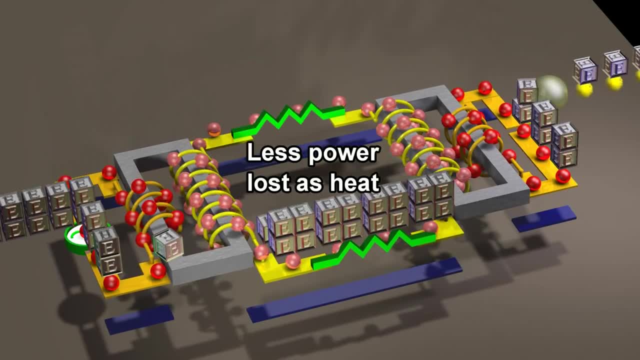 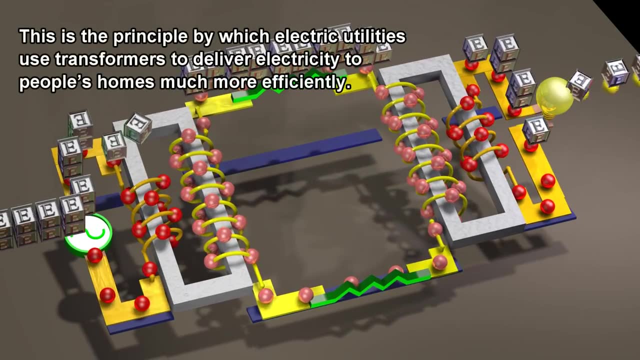 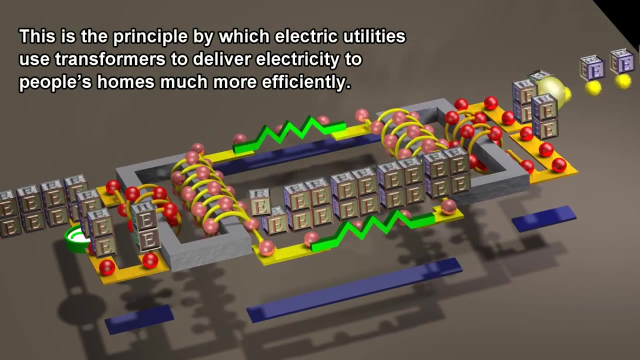 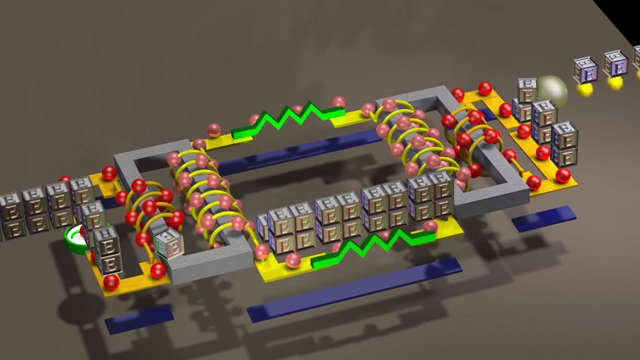 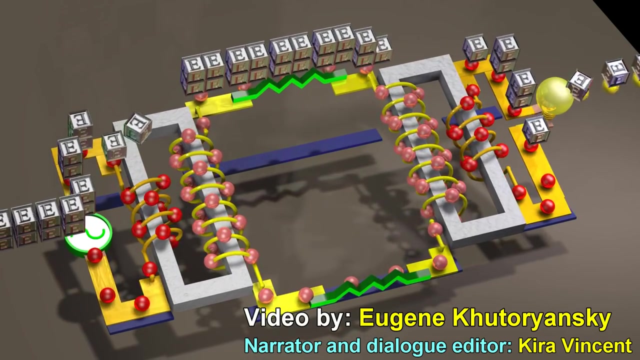 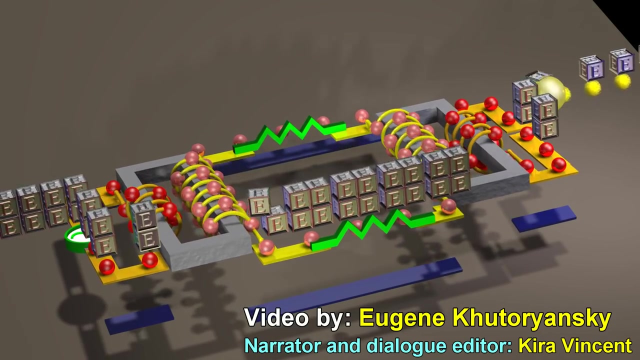 This is the principle by which electric utilities use transformers to deliver electricity to people's homes much more efficiently. Much more information about electricity is available in the other videos on this channel, And information about why transformers work the way they do is available in the video titled Electromagnetism- Maxwell's Laws. Please subscribe for notifications when new videos are ready.